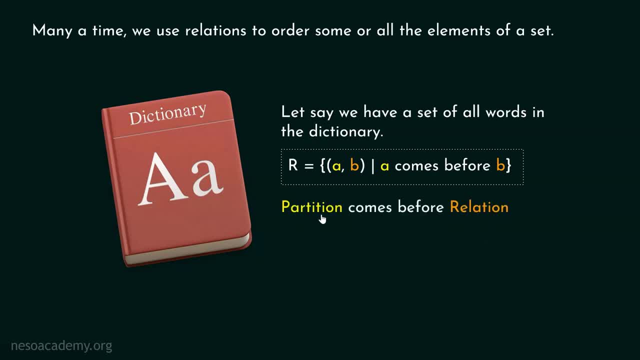 the dictionary, Isn't that? so Here you can see the example. We know that partition, this word partition, comes before this word relation. Why is that? so We can see the first letter of these two words right And compare them. You can see that here we have P. 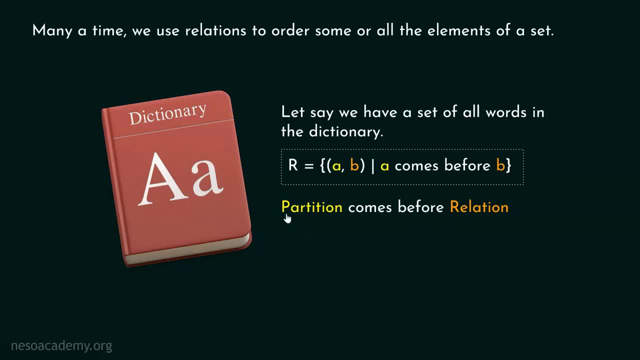 and here we have R right. We know that P comes before R. Therefore partition comes before relation. So we can form an ordered pair of this form, That is, partition comma, relation, right Here, obviously partition comes before relation. 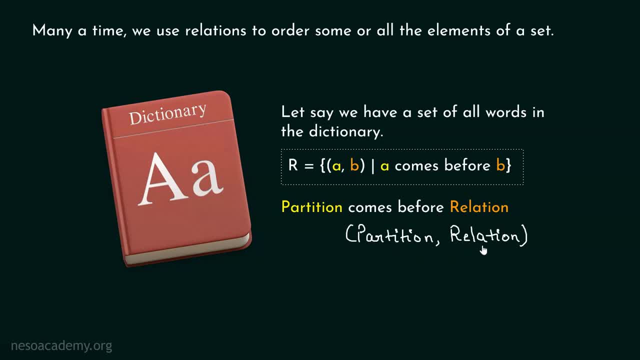 That is why partition is placed before relation in this ordered pair right. It is not the case that relation comes before partition. Therefore we do not have an ordered pair relation comma partition right. So this relation is helping us in ordering all the words in the dictionary right. 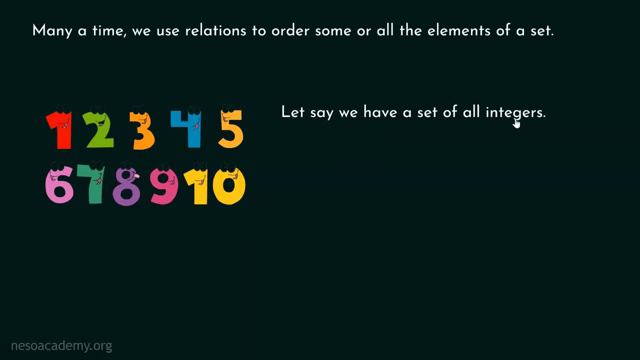 Let's see one more example. Let's say we have a set of all integers. Let's say we are available with a set of all possible integers And we have a relation. and we have a set of all possible integers, And we have a relation R, which consists of all ordered pairs A- B, such that A is less than B. 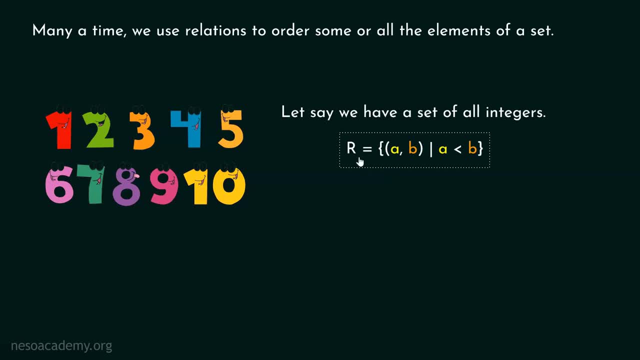 If you closely observe this relation, then you can find that this relation is also helping us in ordering all integers, That is, forming the sequence of integers, where the first integer is less than the second and second integer is less than the third, and so on, right. 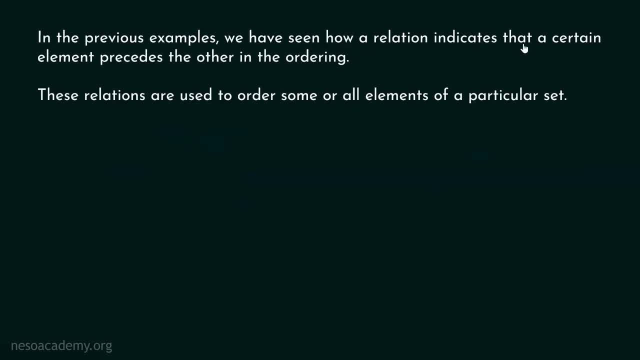 In the previous examples we have seen how a relation indicates that a certain element precedes the second. So we have a relation R which consists of all ordered pairs A- B, such that A is less than B. If you closely observe this relation, then you can see that a relation indicates that a certain element 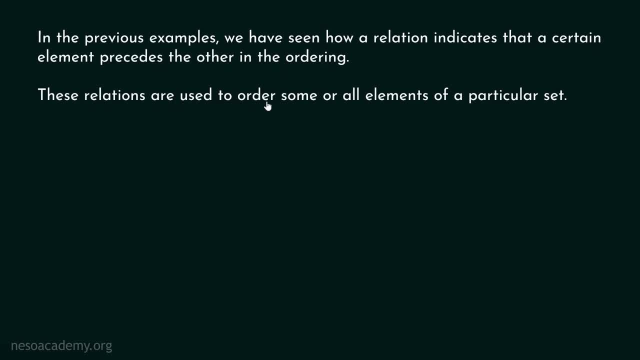 precedes the other. in the ordering right, These relations are used to order some or all elements of a particular set. We know that R1 is helping in ordering all words in a dictionary and R2 is helping in ordering all integers right Here. obviously, ordering depends on these conditions. 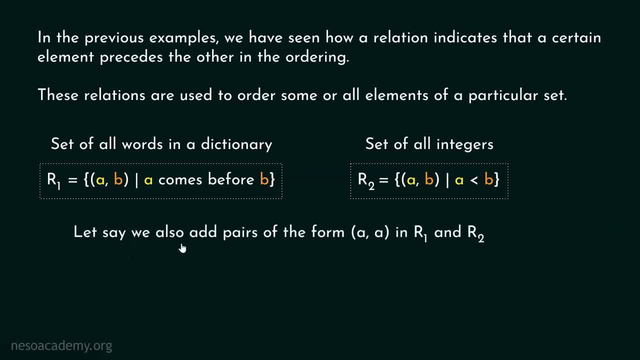 that we have specified right Now. let's say we also add pairs of the form A, A in R1 and R2.. Currently there are no such pairs possible in these two relations. But let's say we add all the pairs of the form A A in R1 and R2 and the relation so 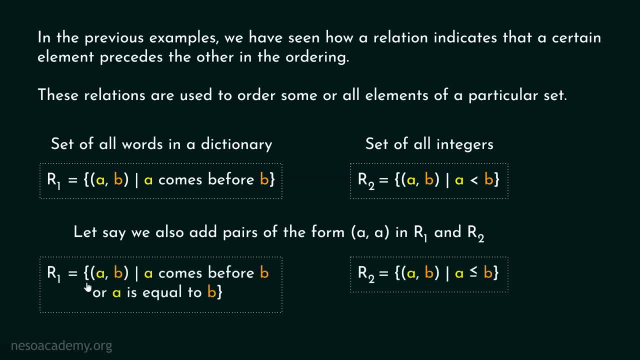 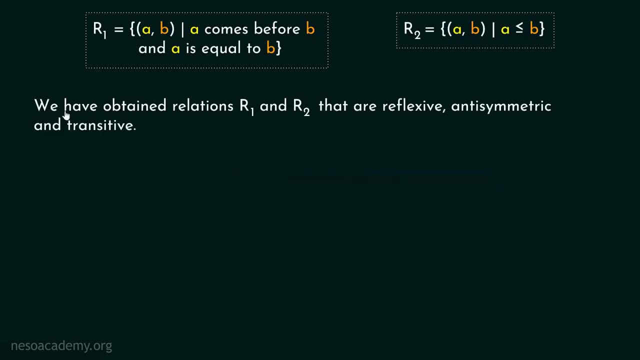 obtained will look like this: R1 must consist of all ordered pairs A- B such that A comes before B or A is equal to B, and. R2 must consist of all ordered pairs A- B such that A is less than or equal to B. 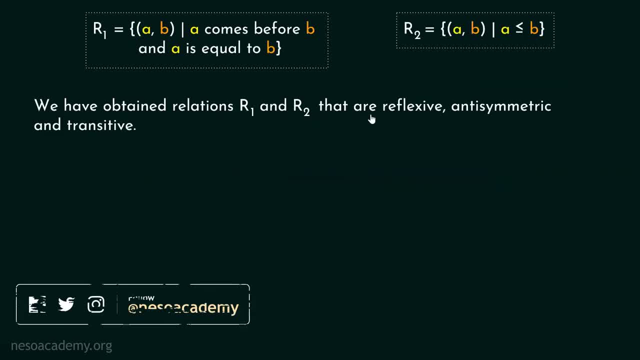 So we have obtained relations R1 and R2 that are reflexive, anti-symmetric and transitive. If you closely observe these relations, then you can find that these relations are reflexive, anti-symmetric and transitive. Why is that so? 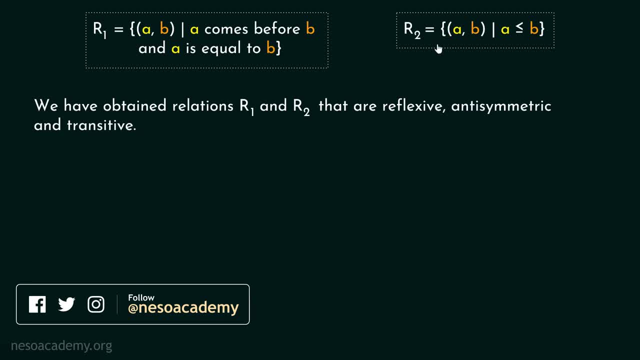 Obviously, these relations are reflexive because we have added the pairs of the form A- A. Apart from this, these two relations are anti-symmetric as well, because ordering is there, right? Right, When we say A comes before B, then it is not the case that B comes before A right. 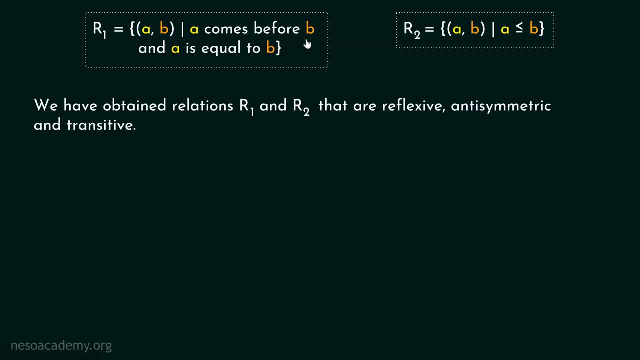 When we say that partition comes before relation, then we cannot say that relation comes before partition. So obviously this relation is not symmetric, This relation is anti-symmetric. Apart from this, this relation is also anti-symmetric because here we are saying A is less than B. 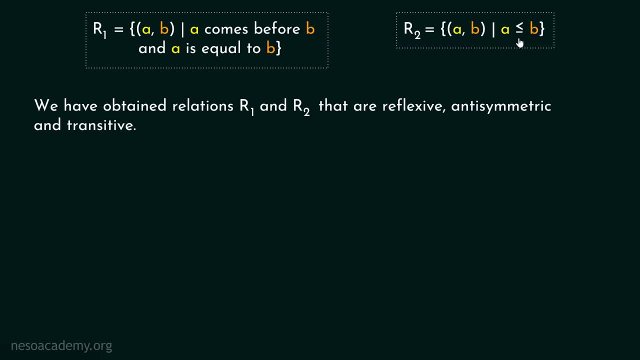 When we say 1 is less than 2,, we cannot say that 2 is less than 1, right? So these two relations are anti-symmetric. Apart from this, these two relations are transitive as well. You can check this on your home. 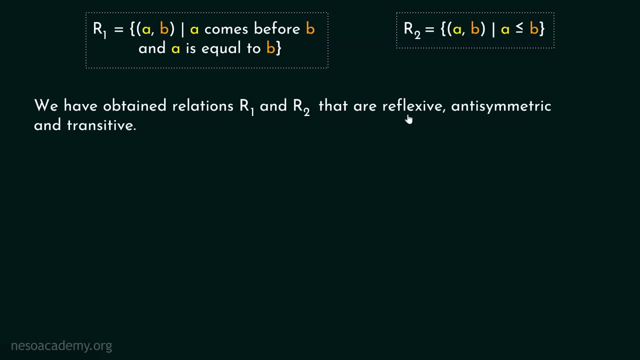 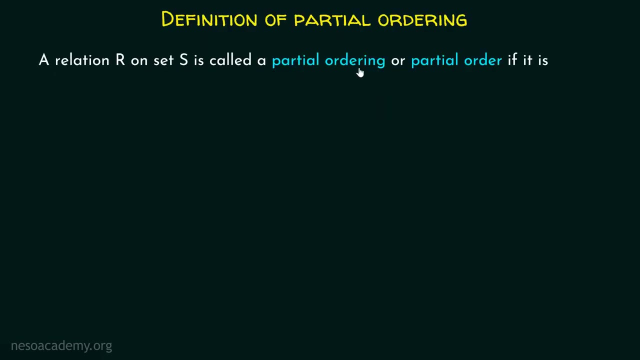 So we can clearly say that R1 and R2 are reflexive, anti-symmetric and transitive. Now it's the high time to understand the definition of partial order or partial ordering. A relation R on set S is called a partial ordering or partial order if it is reflexive. 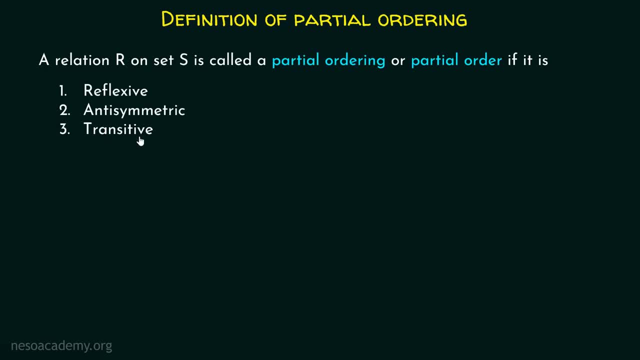 anti-symmetric and transitive. A relation R on set S. this relation is defined on some arbitrary set S and this relation is called a partial ordering or partial order if it is reflexive, anti-symmetric and transitive. The only difference between a partial order and an equivalence relation is that in case 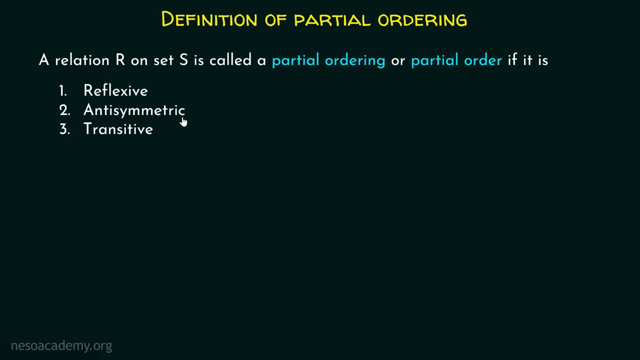 of equivalence relation. we have symmetric property and not anti-symmetric property. Rest of the properties are similar. Right, Let's now understand what these properties mean to us. Reflexive means: each element must be related to itself. We already know this. 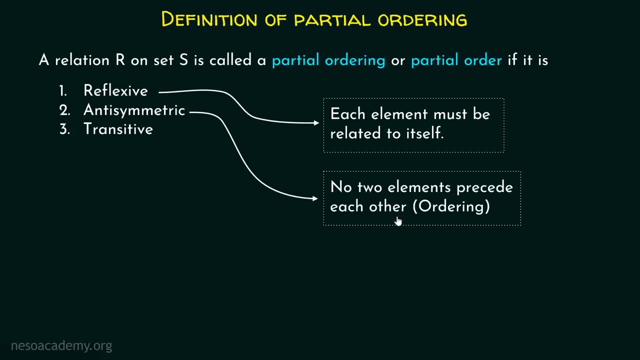 Anti-symmetric means no two elements precede each other. This is important right. This property is helping us in ordering the elements. No two elements precede each other means ordering right, Forming the sequence. Transitive means first element related to second and second element related to third. 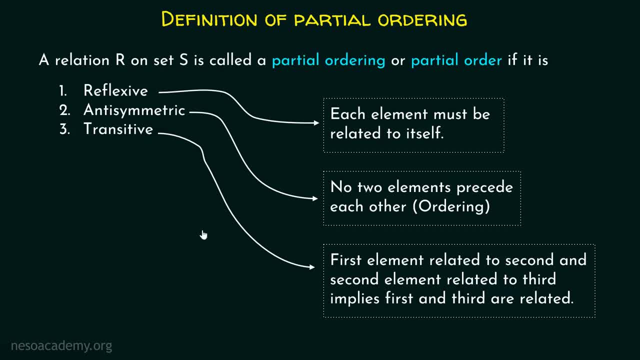 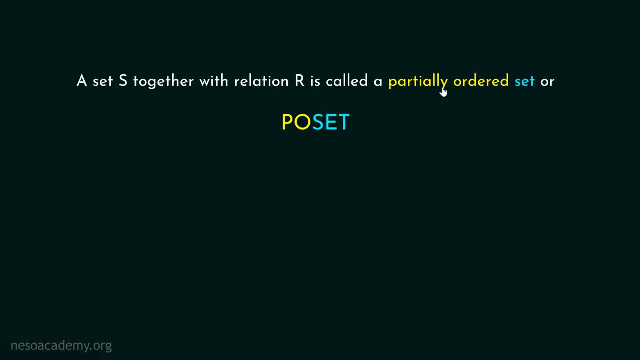 It implies first element related to second. First element related to second implies the first element and third are related. This is what transitive property is all about. Now, a set S together with relation R is called a partially ordered set or post set. Very, very important A set S. 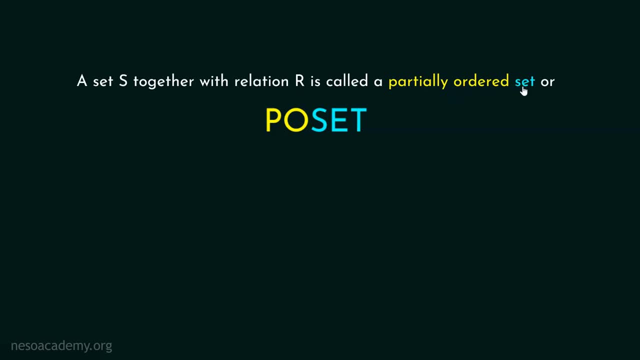 together with relation R, is called a partially ordered set, or we can also say that it is a post set. Obviously it is a short form of partially ordered set. Here P means partially, O means ordered and this set means set. It is denoted by S comma R, or sometimes we use this symbol to denote. 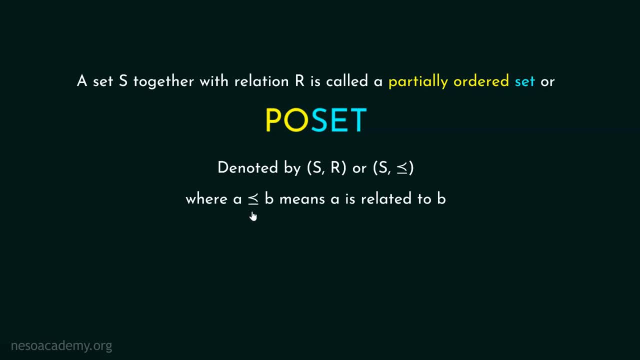 relation R. It seems like it is a less than or equal to sign right, But it is not. This is not a less than or equal to operator. Actually, it is just a replacement of this relation R. We can also replace this symbol by R. 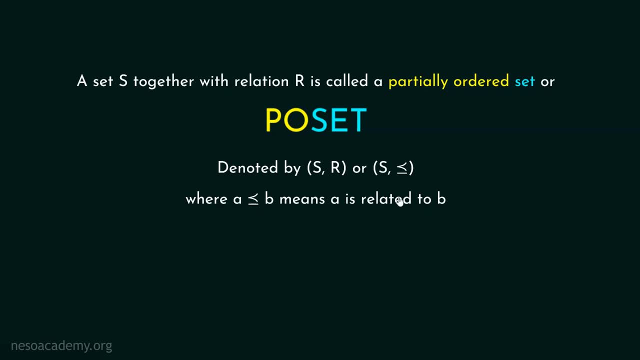 And say A, R. B means A is related to B. We can use these two interchangeably. okay. Here, in place of R, we can use this symbol. They both mean the same. okay, Now let's discuss one example Show. 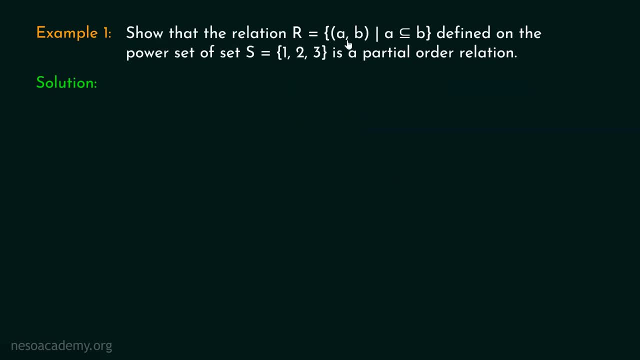 that the relation R, which is nothing but set of all ordered pairs, A, comma, B, such that A is a subset of B, defined on the power set of set S, which is equal to set of all elements like this: 1,, 2,, 3, is a partial order relation. 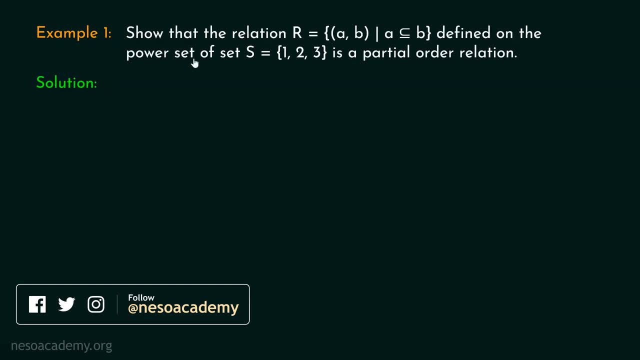 We have to show this- that this relation R, which is defined on the power set of set S, is a partial order relation. Relation R is said to be a partial ordering if, and only if, R is reflexive, antisymmetric and transitive right. We know that we have set S, which consists of these: 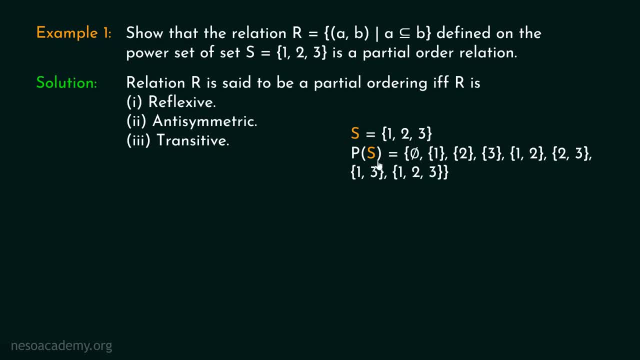 elements 1, 2 and 3.. Power set of set S consists of all these elements. Actually, these are the subsets of this set S. We know power set of set S consists of all these elements. So we have power set of S must consist of subsets of set S. First we have phi, then we have a set with element. 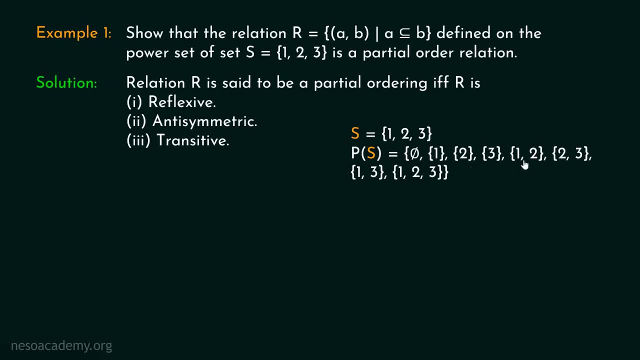 1, set with element 2, set with element 3, then we have a set with these two elements 1 and 2, then we have set with these two elements 2 and 3, set with two elements, 1, 3- and a set with three. 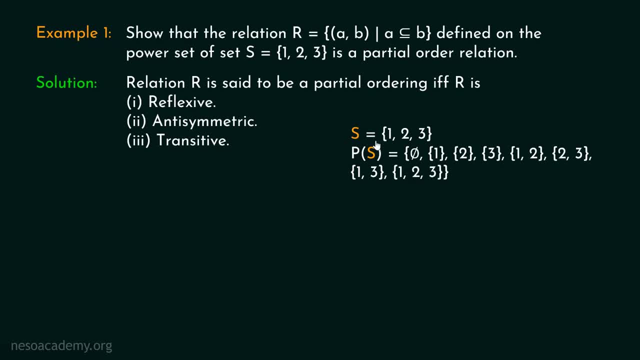 elements 1, 2 and 3.. These are all subsets of this set right, This relation. R is defined on this set, that is power set of set S, And we know that R is nothing but set of all ordered pairs of this form. 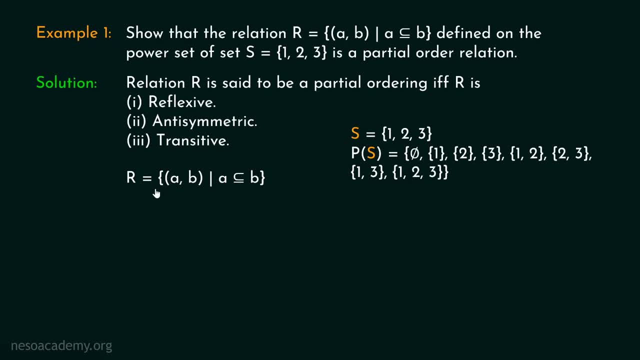 A, comma B, such that A is a subset of B. Now let's see whether this relation is reflexive or not. Let's check the reflexivity property. We know that, according to reflexivity, A must be the subset of A. Here, obviously, A belongs to power set of set S right, And we know that this is true, Obviously. 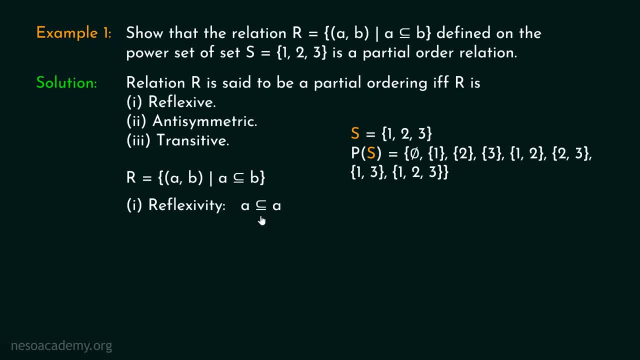 because every element is a subset of itself. Apart from this antisymmetric property says A is a subset of B and B is a subset of A. implies A equal to B. Obviously this is true again If A is a subset of B and B is a subset of A. 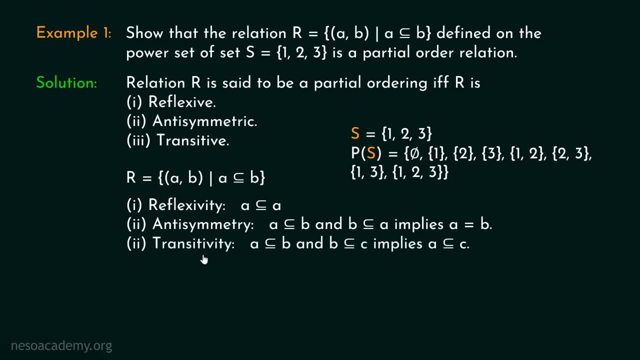 then obviously A must be equal to B. We know according to transitivity: if A is a subset of B and B is a subset of C, then obviously A must be a subset of C. This is also true, So it is clear. 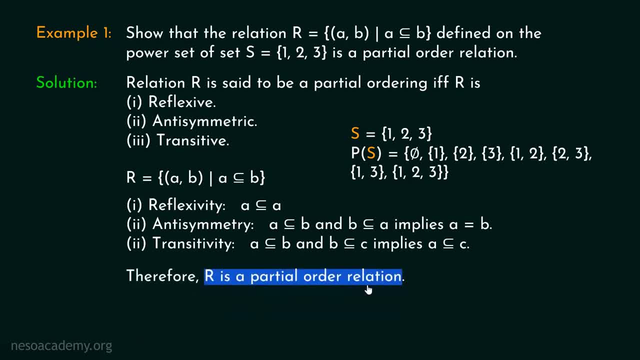 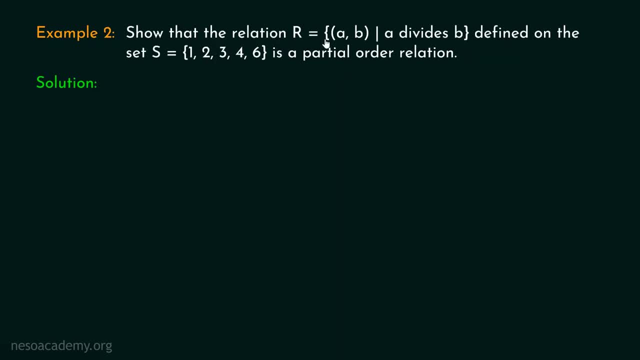 that this relation is a partial, Isn't that? so Now let's see example 2.. Show that the relation R, which is equal to set, of all ordered pairs A, comma, B, such that A divides B, defined on the set S, which consists of 5 elements. 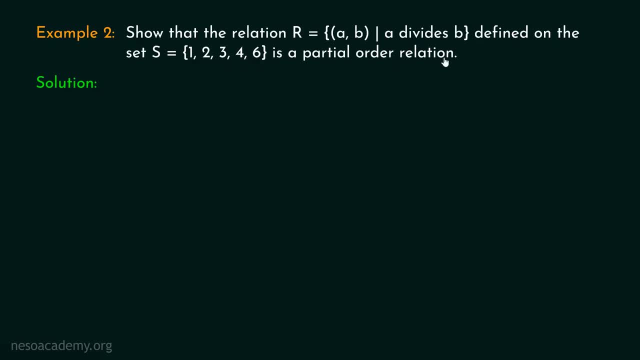 1,, 2,, 3,, 4 and 6 is a partial order relation For this. we know that relation R is said to be a partial ordering if, and only if, R is reflexive, antisymmetric and transitive. We know that we. have this relation R, which consists of all ordered pairs, A, comma, B and B is a subset of B. So this is true again, If A is a subset of B and B is a subset of C, then obviously A must be a subset of A. 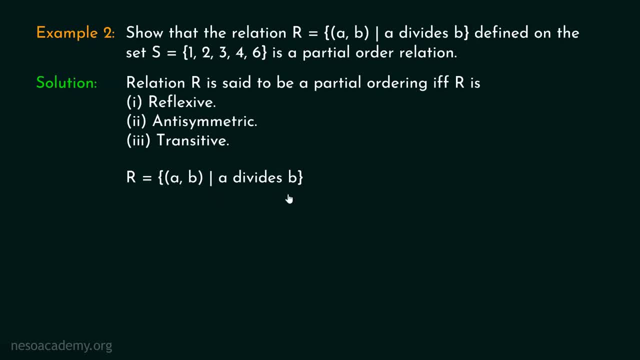 This is true again, If A is a subset of B and B is a subset of C, then obviously A must be a subset of A comma B, such that A divides B. Apart from this, we are available with this set, which consists of total 5 elements: 1,, 2,, 3, 4, 6.. This relation is defined on this set. First we will identify: 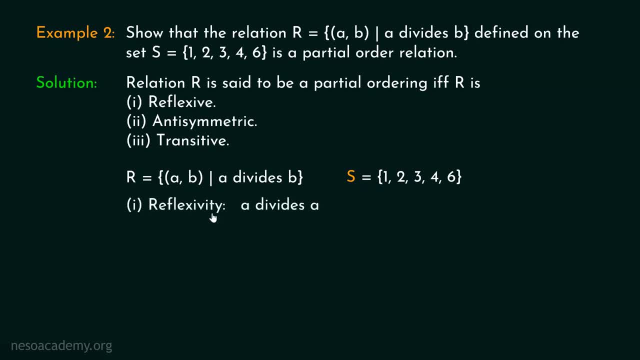 whether this relation is reflexive or not. According to reflexivity, A must divide A. Obviously, it is true, right, A divides A. There is no doubt about this. Apart from this, this relation is antisymmetric. also, If A divides B, then obviously A must be a subset of A. 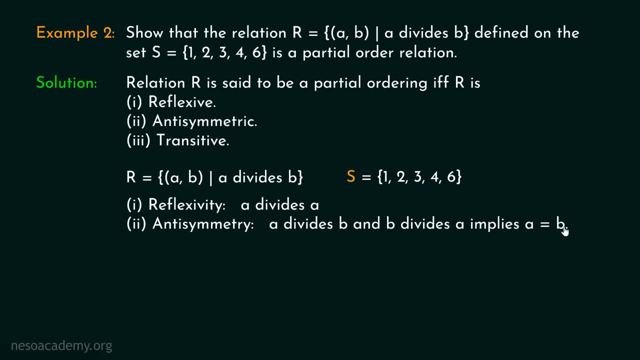 If A divides B and B divides A, then obviously A must be equal to B. This is only possible when A is equal to B. If A divides B and B divides A, then this implies A is equal to B. Let's see one. 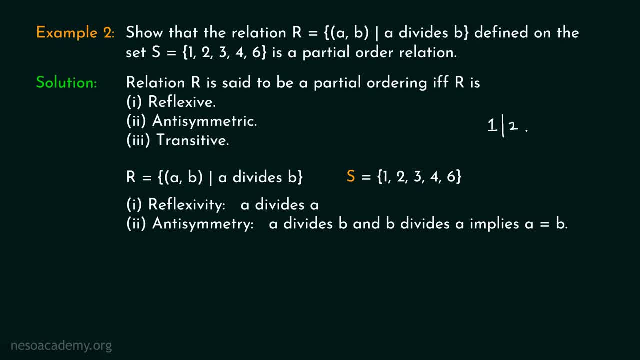 example, We know that 1 divides 2, right, But 2 does not divide 1.. But if we say that 1 divides 1 and 1 divides 1, then obviously they are equal right. That is why it is possible. 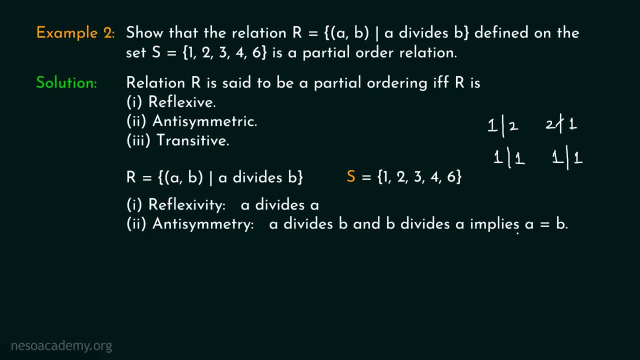 So if A divides B and B divides A, then this implies A is equal to B. right Apart from this, this relation is transitive as well. If A divides B and B divides C, then A divides C. There is no. 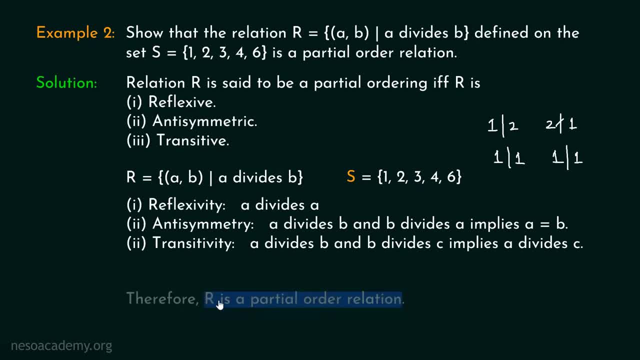 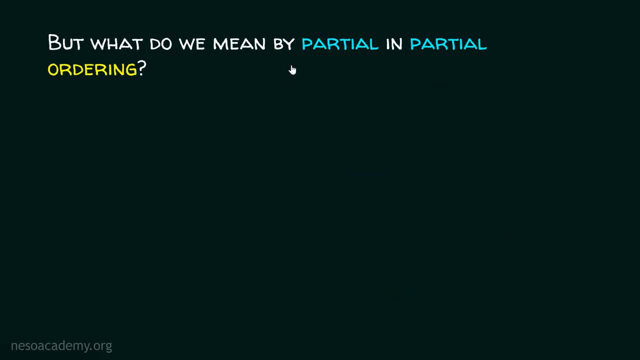 doubt about this. So this relation is nothing but a partial order relation. But what do we mean by partial-impartial ordering? What is the meaning of partial-impartial ordering? What is the meaning of ordering right, But what is the meaning of this partial-impartial ordering? 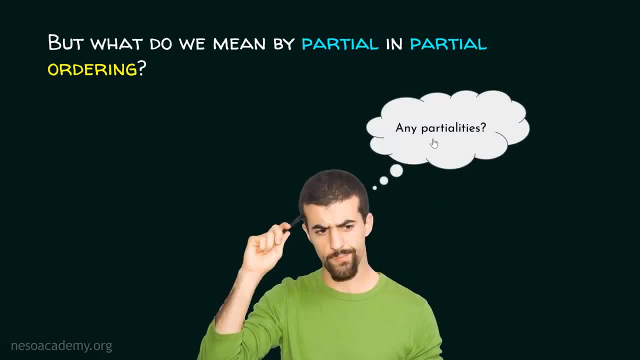 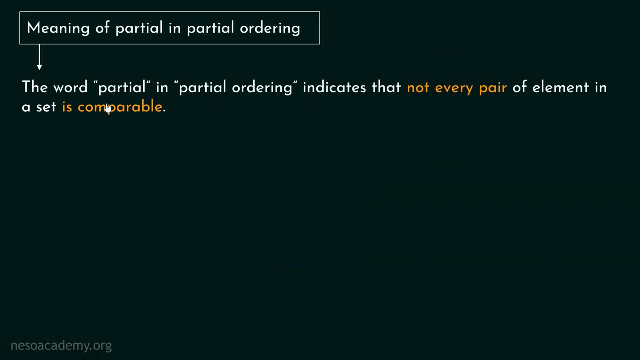 Why we are saying partial ordering. Are there any partialities? The word partial-impartial ordering indicates that not every pair of element in a set is comparable. Okay, that is cool, But what is the meaning of comparable? Now let's just try to understand the difference between comparable. 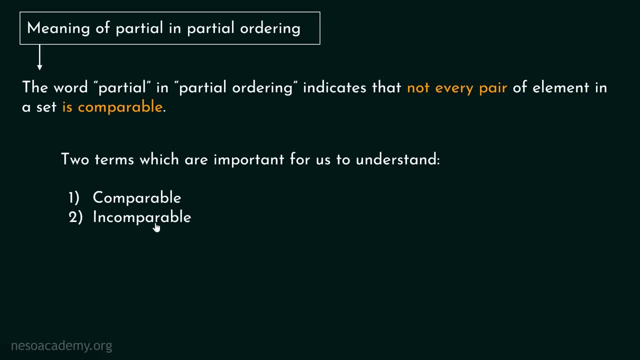 and incomparable. This will help us in understanding what do we mean by comparable and incomparable. Here we are saying: the word partial-impartial ordering indicates that not every pair of element in a set is comparable, Not every pair, okay. That is why partial comes in, partial ordering. 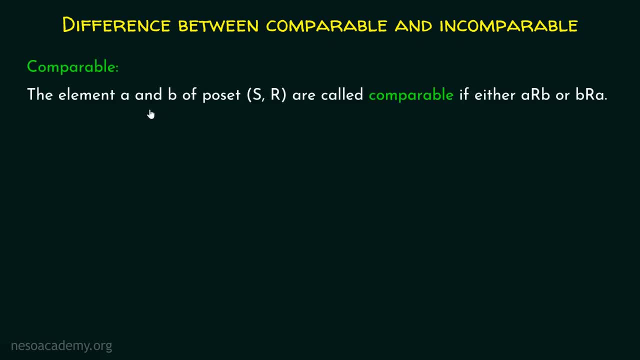 Let's understand the difference between comparable and incomparable. The element A and B of poset S R are called comparable if either A is related to B or B is related to A Simple right: The element A and B. we are talking about two elements of poset S R. 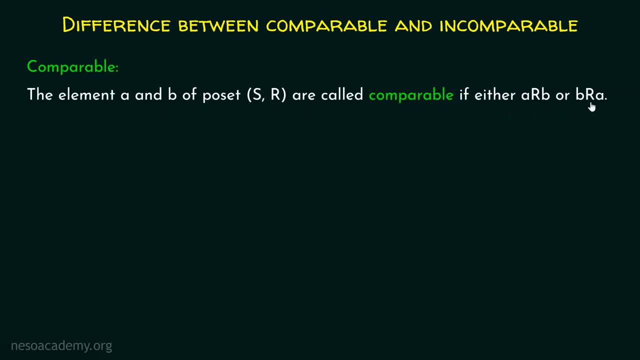 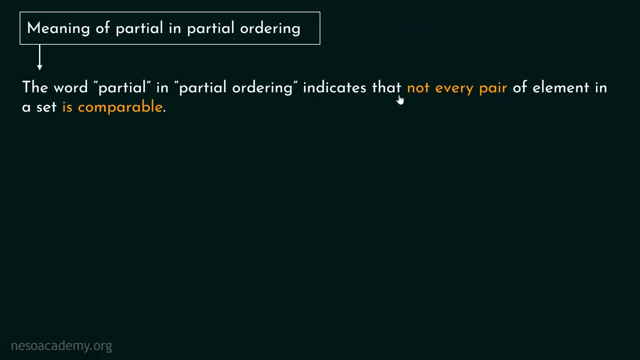 They are called comparable if either A is related to B or B is related to A, And the element A and B of poset S R are called incomparable if neither A is related to B nor B is related to A. So here the word partial is quite justified, because we are saying that not every 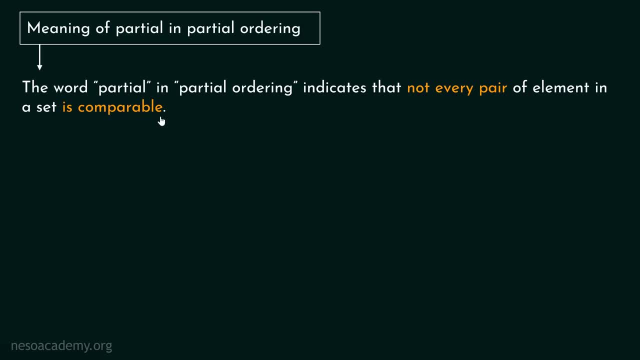 pair of element in a set is comparable, right, Some relation is defined on a particular set. That relation is called partial order, because not every pair of element in a set is comparable. okay, This means we cannot say that every element is related to each other. 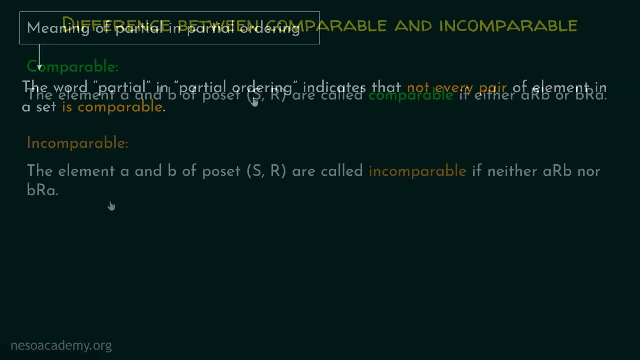 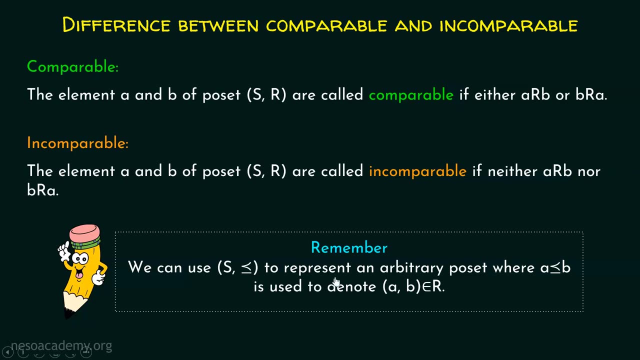 okay, That is why we are using this word partial in partial ordering. Now, please remember, we can use S R. we know this: that this symbol represents relation R to represent an arbitrary poset where A R, B is used to denote A, B belongs to R. 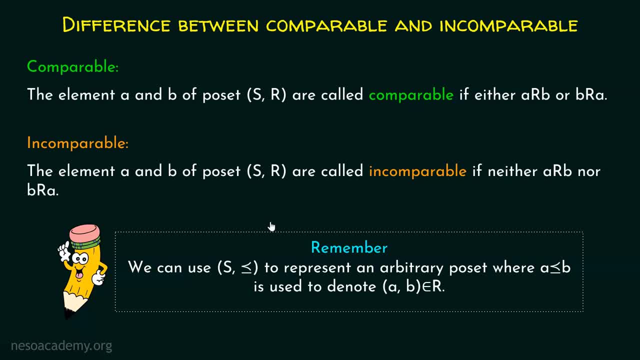 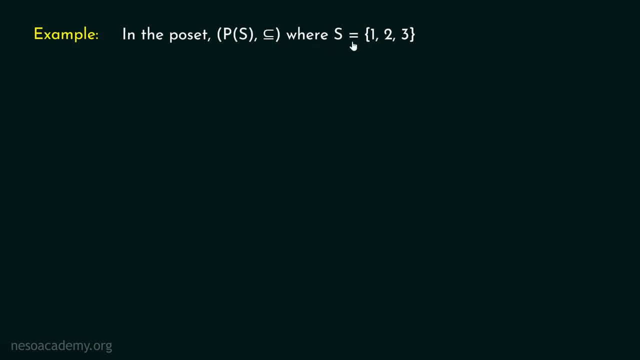 Now let's discuss one example related to comparable and incomparable elements In the poset P S. this subset, where S is equal to 1, 2, 3,, 1, 3, this set is not subset of 2 or this. 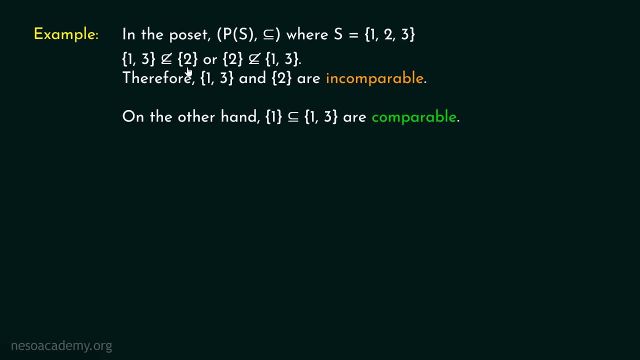 set is not subset of this set. This set is not subset of this set, or we can say that this set is not subset of this set. Therefore, we can say: this set, which consists of two elements- 1, 3- and this set, which consists of just a single element, 2, are incomparable right. 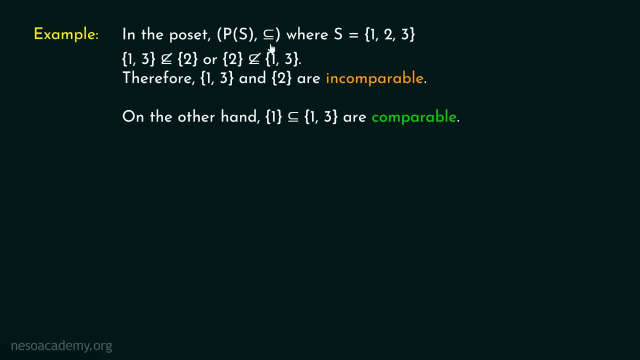 Obviously, we know that this is a poset. We have already proved this right Here. you can see, not every element is comparable, right? You can clearly see that this set is not a subset of this set and this set is also not a subset of this set. This means that this set. 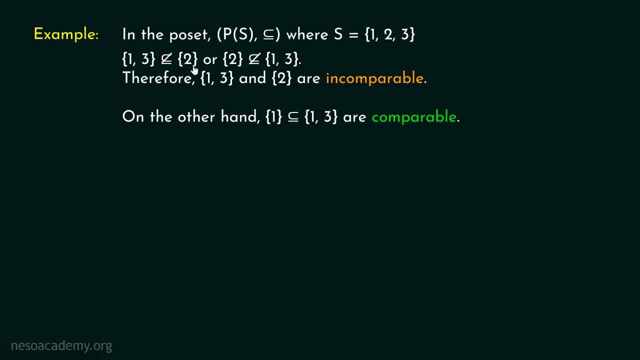 which consists of two elements, 1, 3, is not related to this set, which consists of single element 2.. Therefore, these two elements are incomparable right. On the other hand, this set is a subset of this set. Therefore, we can say these two elements are incomparable right.